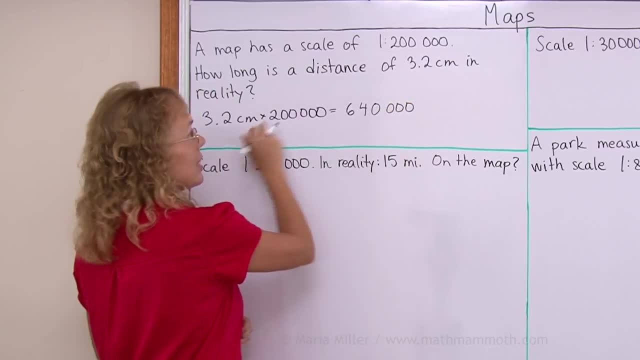 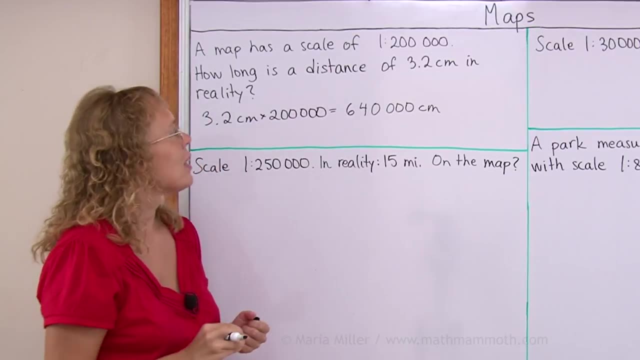 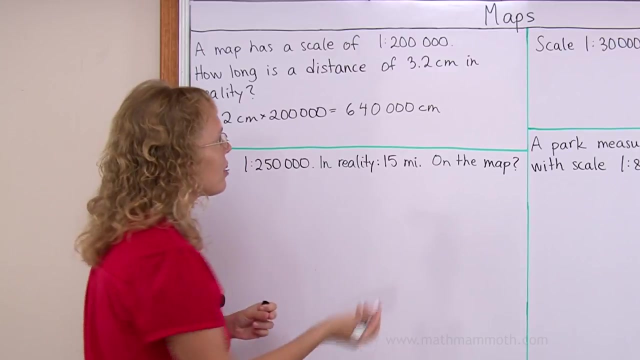 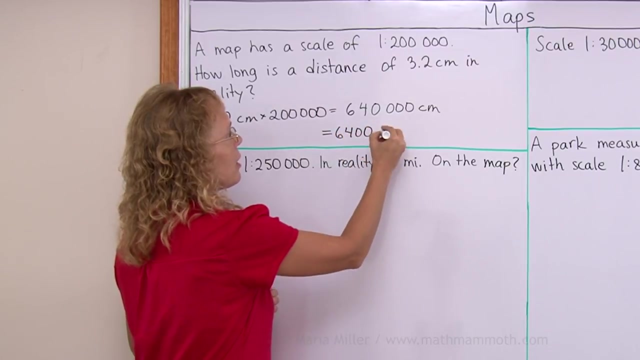 So 640,000 centimeters. But of course you don't want to give that distance in centimeters. you want to convert that And let's first change it into meters, remembering that 100 centimeters makes a meter. So I drop two zeros, I divide by 100 and I get this many meters. 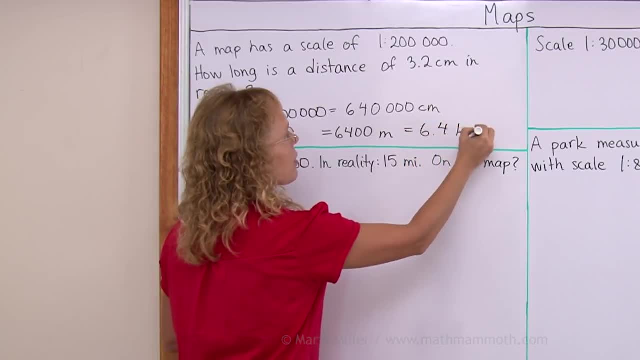 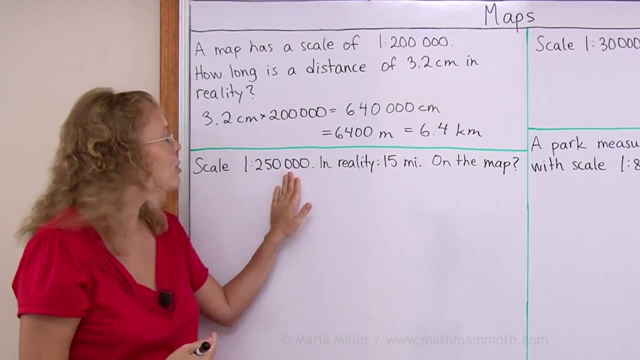 And now into kilometers. we get 6.4 kilometers Over here. the map has a scale of 1 to 250,000. And we have a distance that in reality measures 15 miles. And how long would it be on the map? 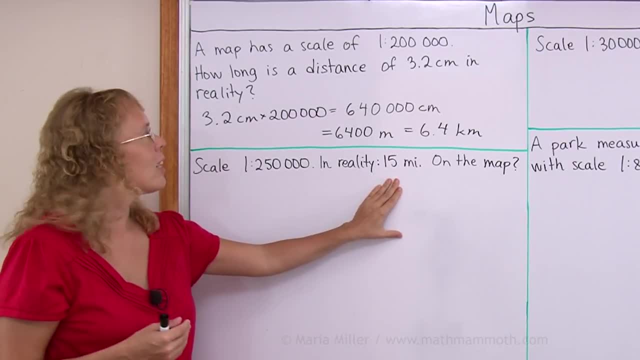 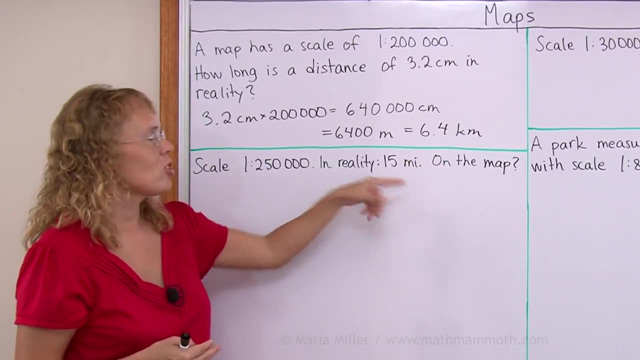 Now this is a little bit more complicated. It's a more complicated calculation than what we had here, because it is customer units, it's not metric units. We need to change miles into feet, into inches, because on the map you want to tell somebody. 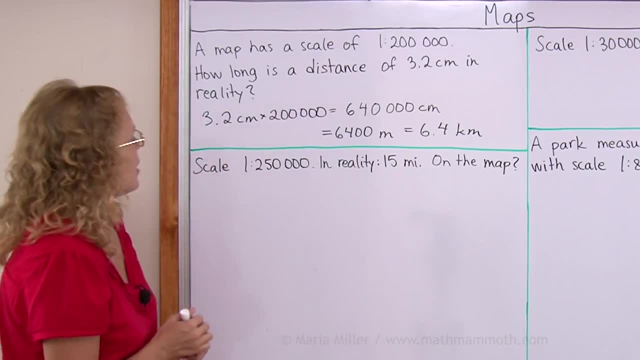 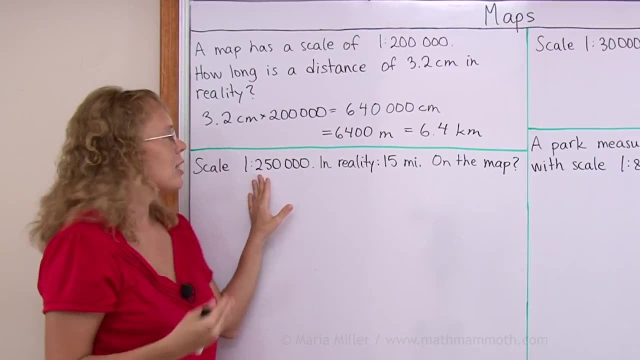 that. okay, it's going to be so many inches on your map, So, but the basic idea is the same: that one unit on the map corresponds to 250,000 units in reality, And so each time when we are converting, we either multiply by this: 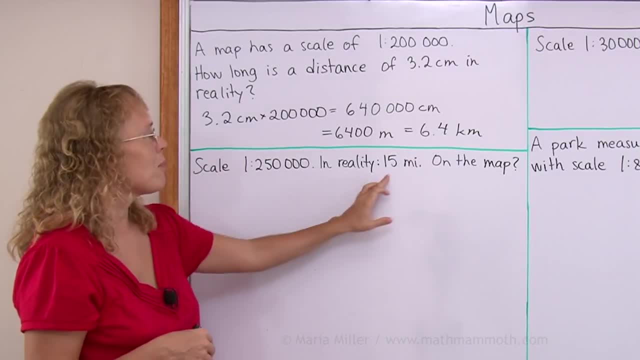 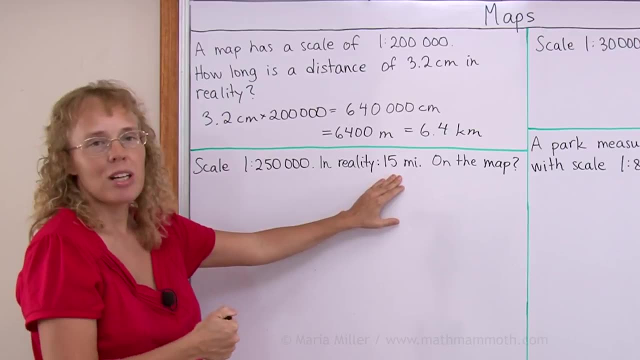 Or divide by this big number, And this time, of course, we have to divide, so we get a really small number. Okay, We wouldn't want to multiply this by 250,000, we would get a huge amount of miles. 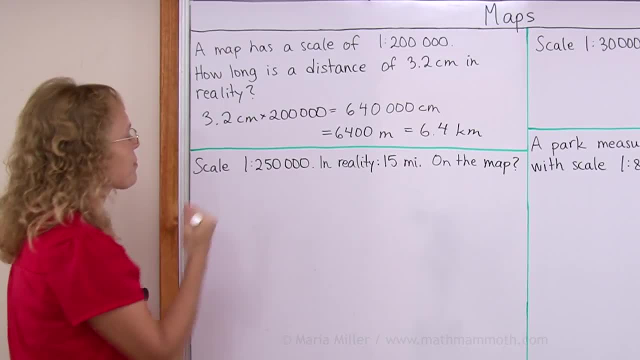 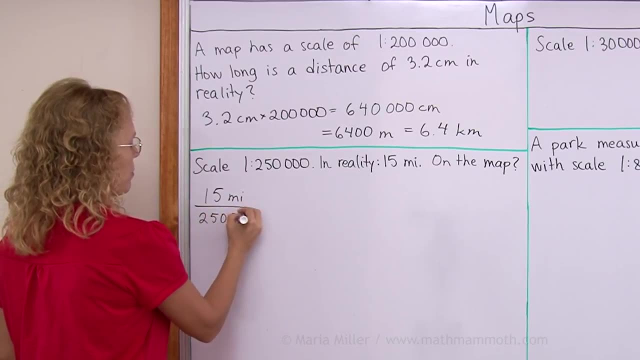 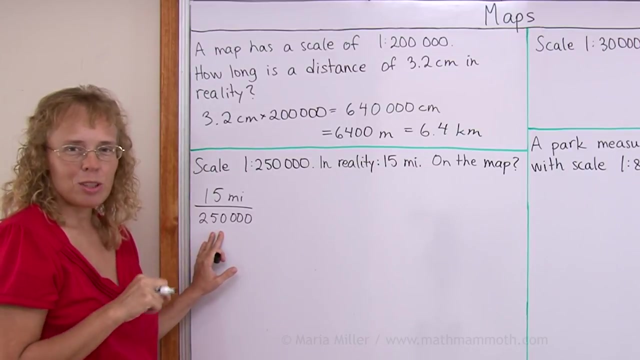 So we divide 15 miles by 250,000.. And I'll show you two ways to do this. All this conversion. Now you can put this into a calculator And you will get some really small numbers, Really small decimal numbers: 0.00, something, okay. 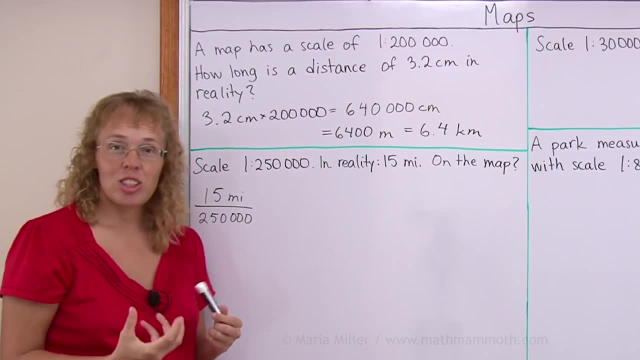 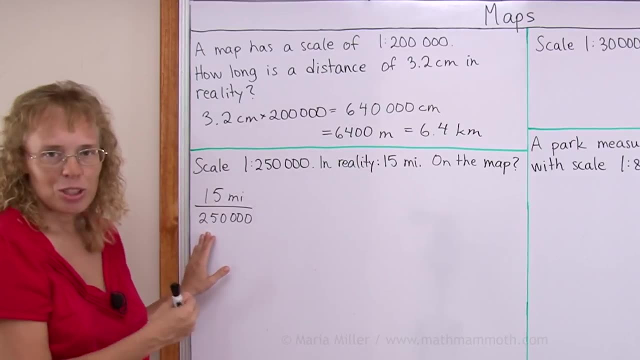 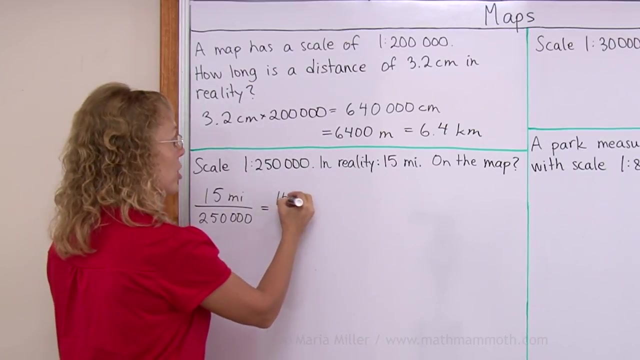 So instead I could first change those 15 miles into so many feet and then into so many inches And then only lastly divide by 250,000.. So if I do that, I will just work with this 15 miles here on top and change that into. 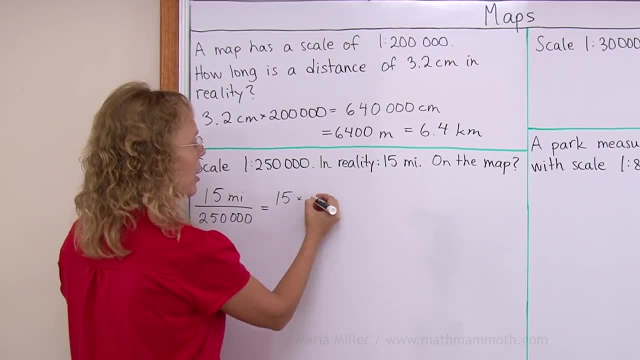 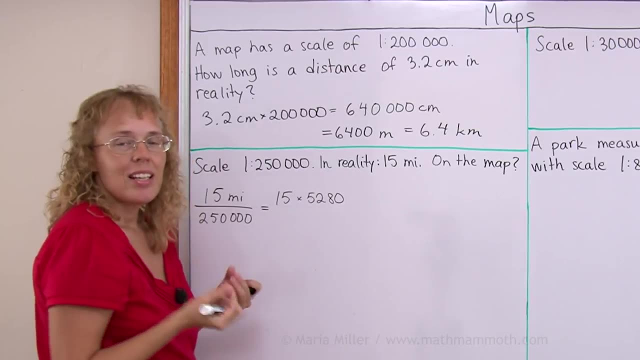 feet. First of all, if I want to change it into feet, I will multiply it by 5,280.. Right, And this would tell me how many feet it's gonna be, And then I will change that into inches. This is however many feet it is. 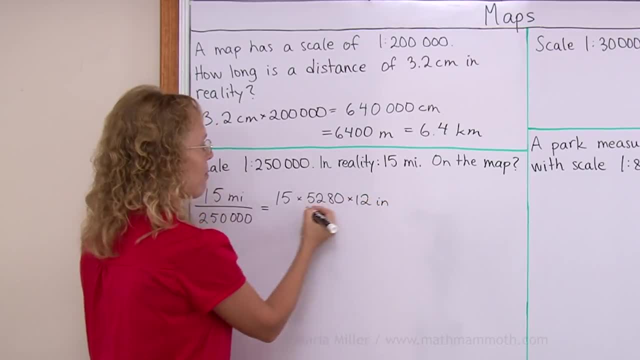 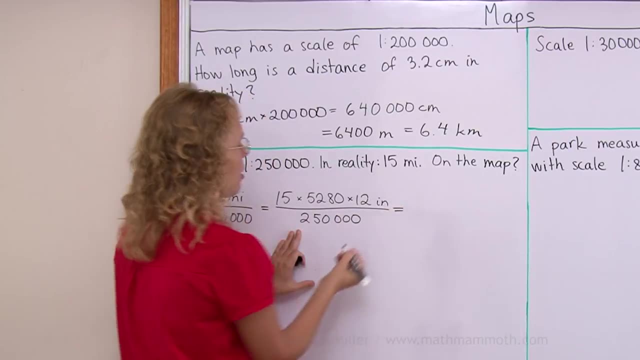 I multiply that times 12 to get how many inches it would be, And now the division by 250,000.. And this will now give me the amount in inches. So I would first multiply in a calculator using a calculator and then divide by this. 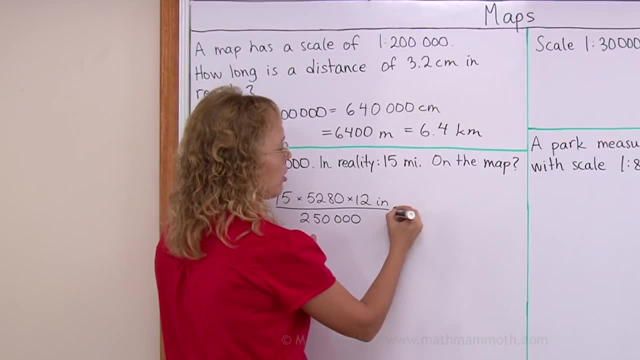 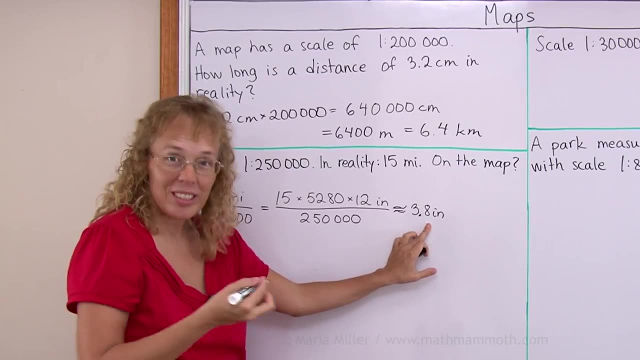 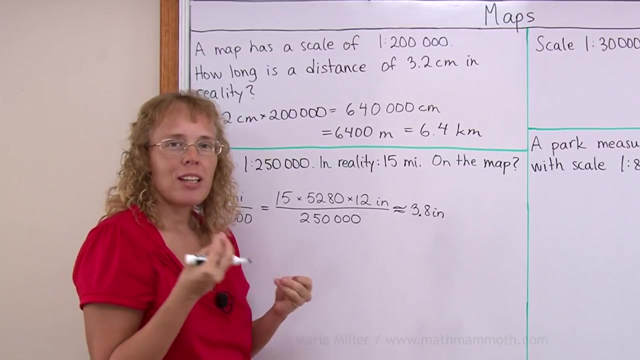 number And the answer is Okay, it's approximately 3.8 inches. And if you don't want to give it as 0.8, you know 3.8 inches- then you would need to change the 0.8, or 8 tenths into maybe 8 parts of an inch or 16 parts of an inch. 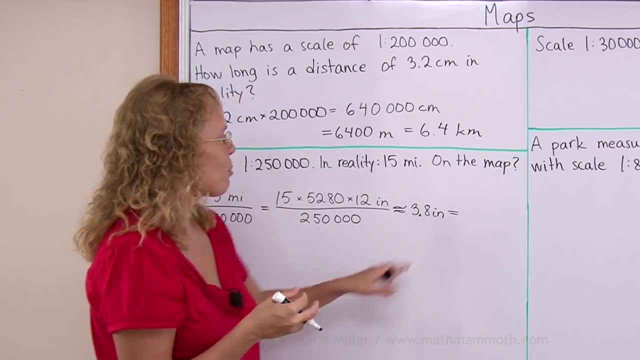 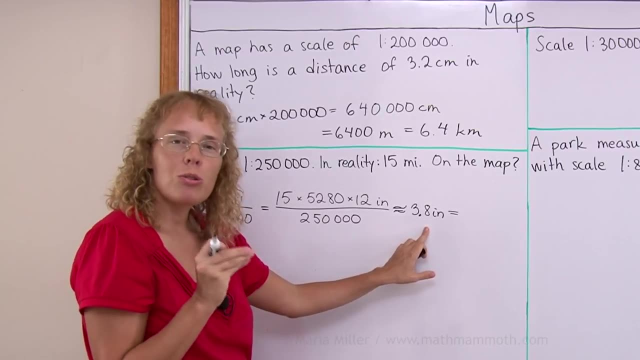 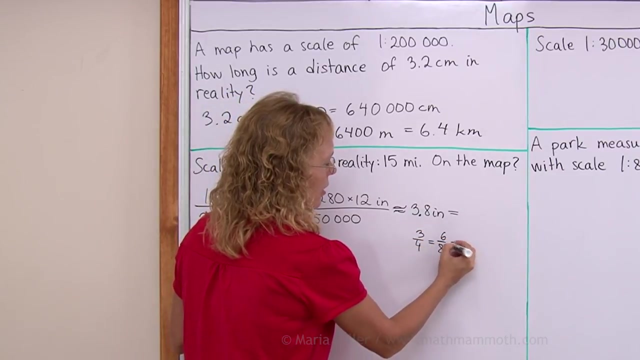 And that can be a matter of trial and error. For example, you might check 3 fourths of an inch. well, that would be 0.75.. And check anything that's close to 3 fourths of an inch. For example, 3 fourths is the same as 6 eighths is the same as 12 sixteenths parts of an inch. 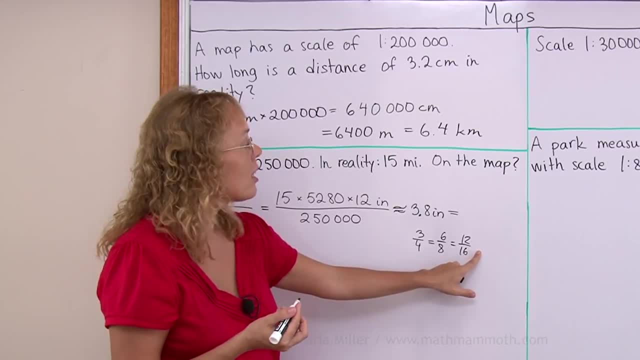 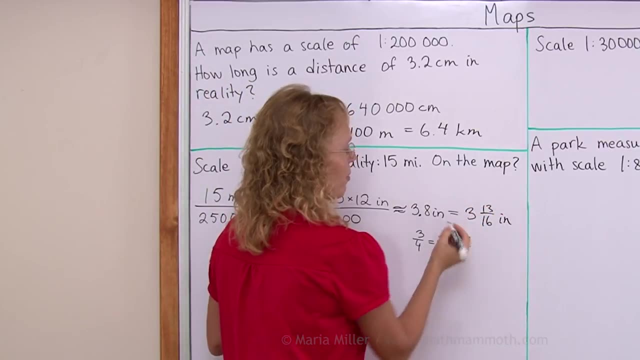 And if you try this and if you try the next one, 13 sixteenths, then that is pretty close to that decimal. So this would be 3 and 13 sixteenths of an inch, or it is close to it. 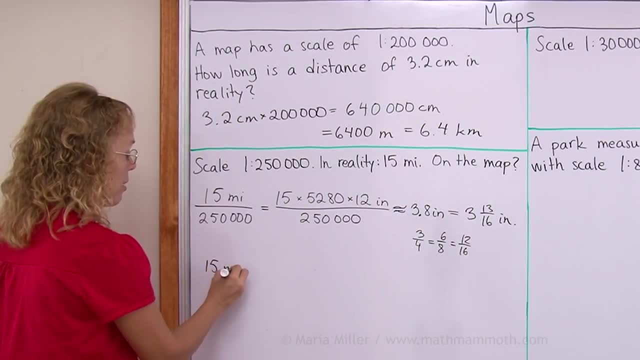 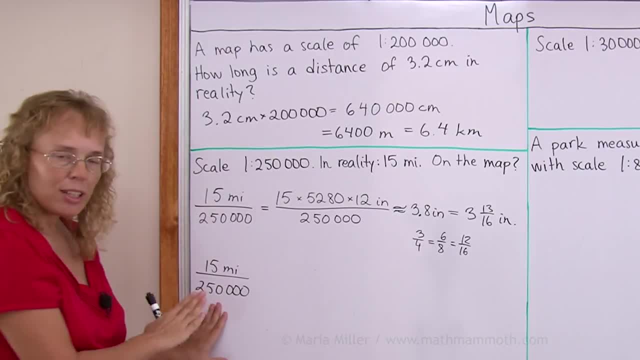 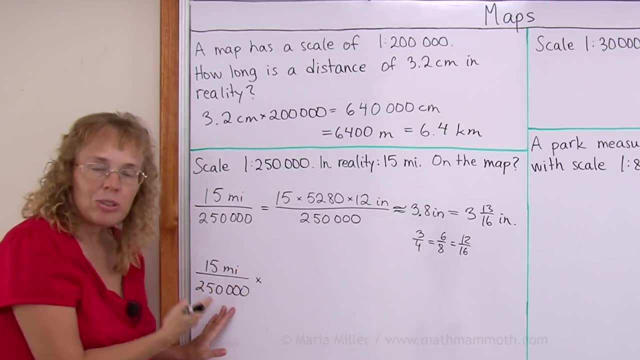 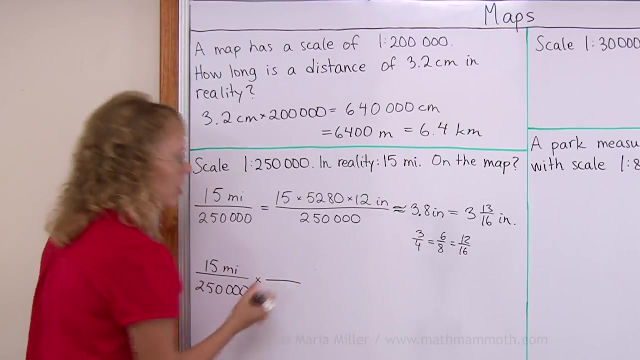 And this would give me a decimal number. but before I calculate anything with a calculator, I will then put the conversions here. Okay, This will give me an amount in miles. I want to convert that into feet, and then I will use the ratio of 5280 feet to 1 mile. 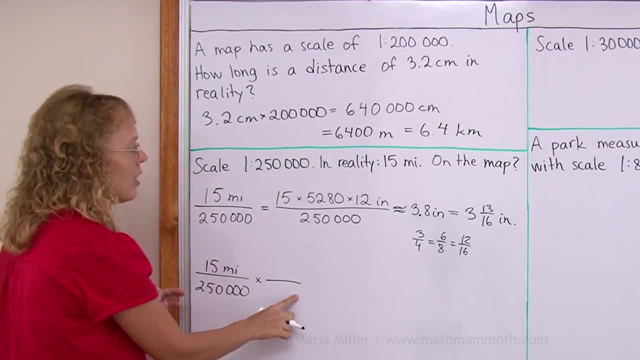 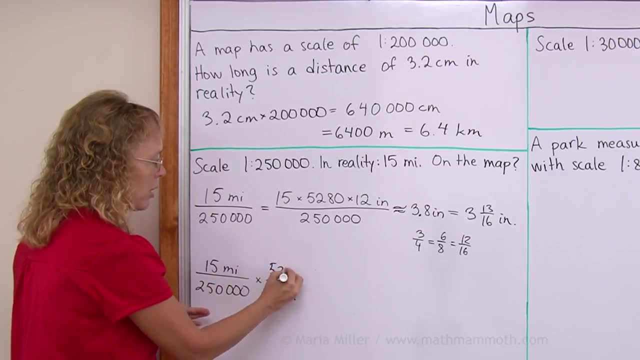 I either write the feet here and 1 mile here, Or vice versa, And this time I want my miles to cancel, so I put 1 mile here and 5280 feet here. This alone here is a ratio that is equal to 1.. 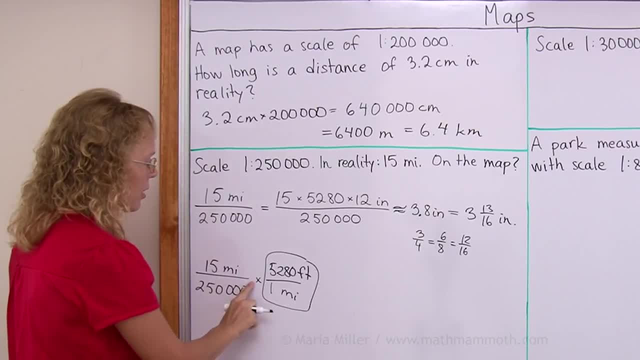 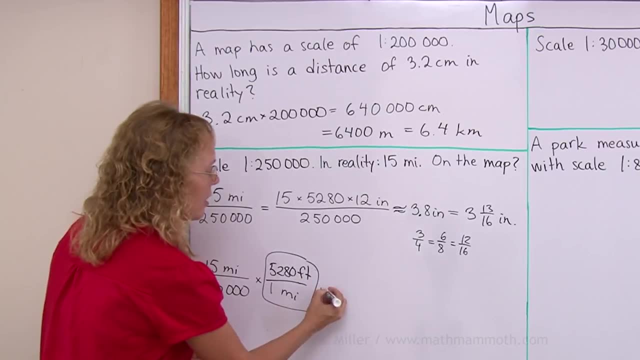 It is equal to number 1.. So I am multiplying this whole thing times 1.. A special form of number 1, yes, but it helps us convert the units. And then the same thing with the 12 inches to 1 foot. 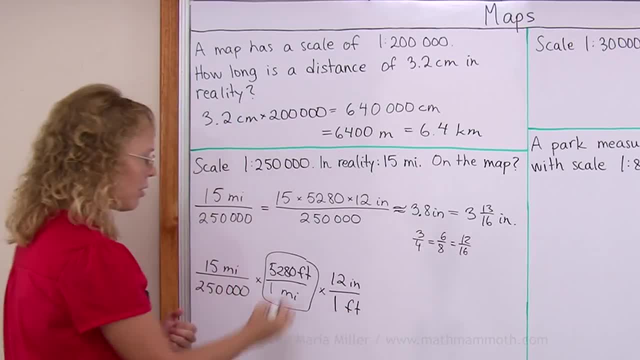 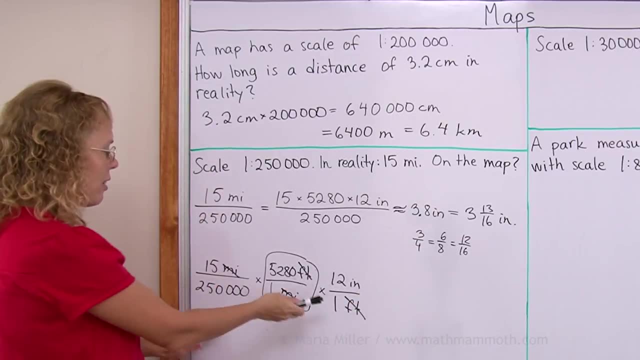 12 inches here, 1 foot here, 1 foot here, So that these feet will cancel and here the miles will cancel and my units will be in inches. And now I have written this out and then I will use the calculator. 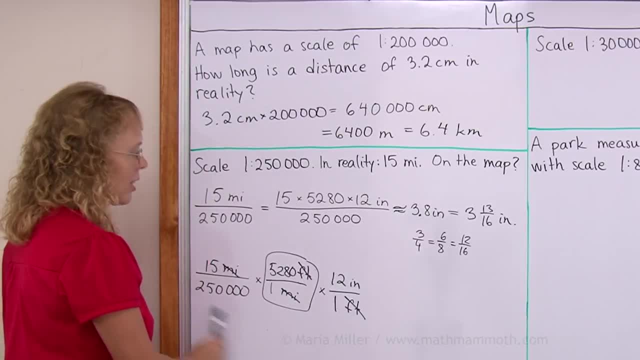 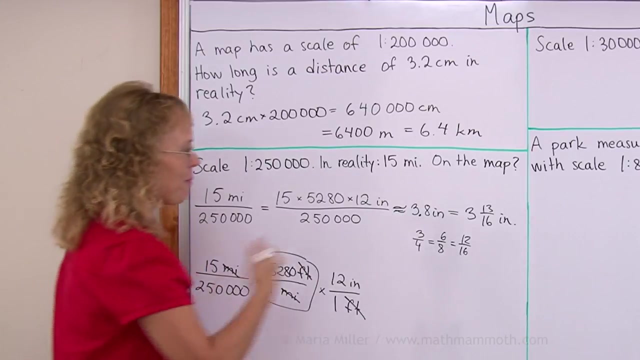 So I can go 15 divided by 250,000, then I go times 5280 times 12.. Or you can alternatively go 15 times 5280 times 12 divided by 250,000. Like we did here. Either way you get the same. 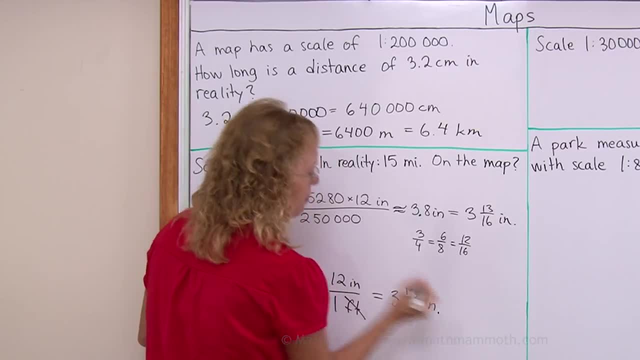 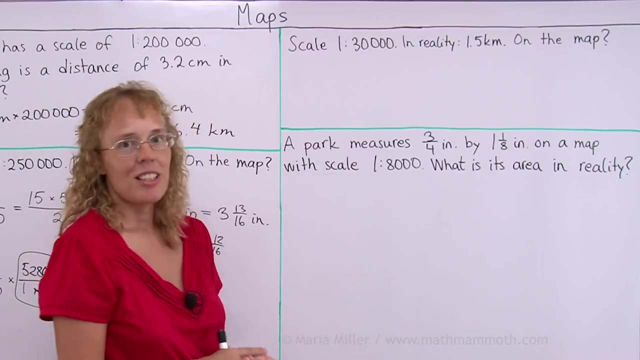 This will eventually be the same: 3 and 13 sixteenths of an inch. Here I have a problem with metric units, so this is an easy problem. Scale is 1 to 30000, and in reality we have a distance of 1.5 kilometers. 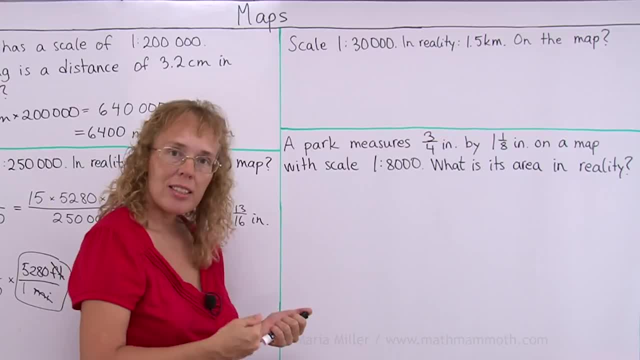 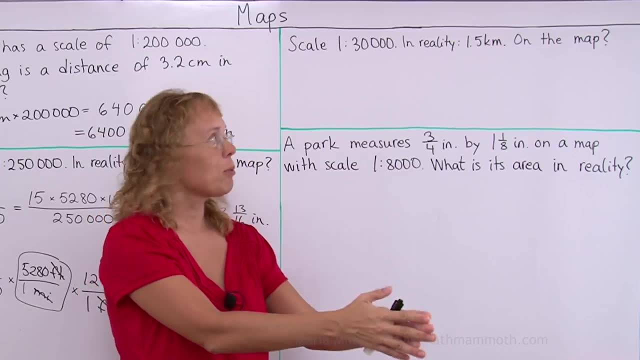 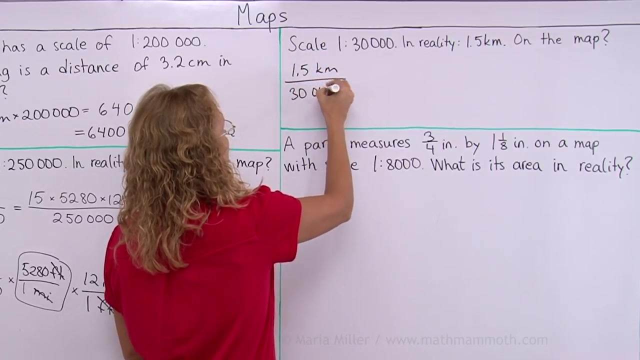 How about on the map? Okay, we are going from reality to the map. So we need to make this distance of 1.5 kilometers, We need to make it smaller. So we will divide 1.5 kilometers, Divide it by 30000.. 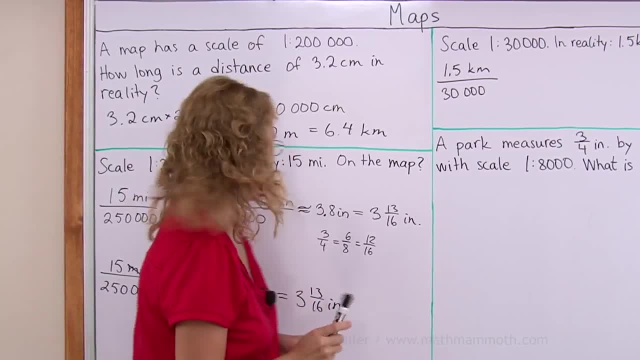 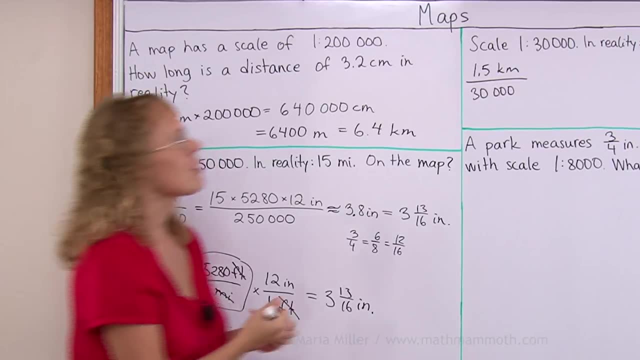 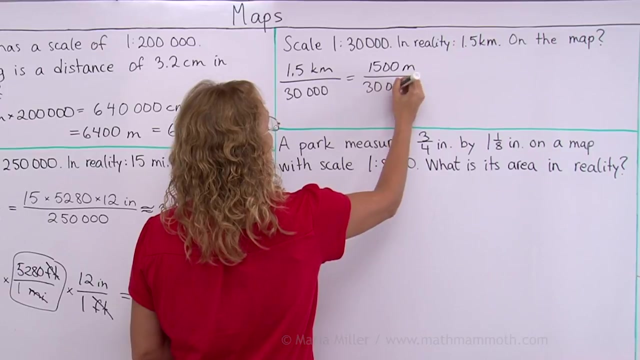 Okay, Now I will do what I did here. I will change the 1.5 kilometers into meters and centimeters, Then divide This- is 1500 meters right- And then into centimeters. I will multiply it by 100. 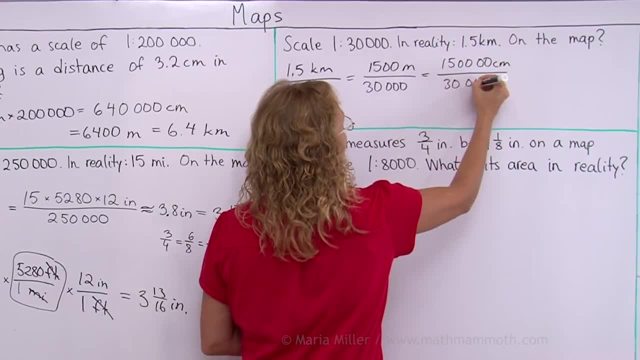 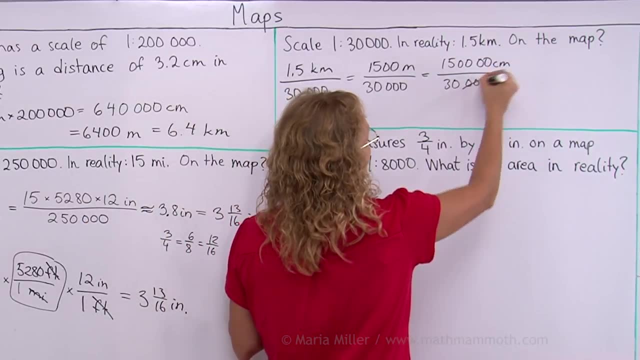 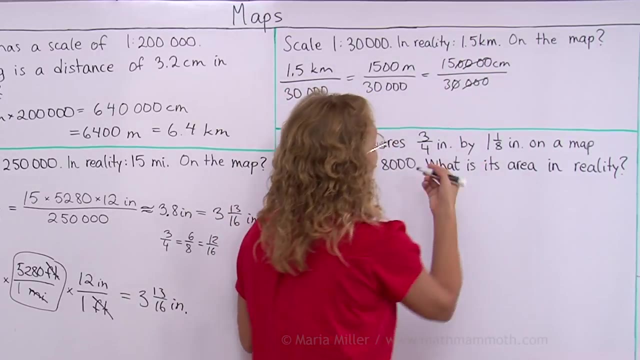 So two zeros there. Now my division will be very easy, because I can just cancel first of all by 10000.. It looks like this: I cancel these zeros out. It means that I divided both by 10000.. And it is just 15 divided by 3.. 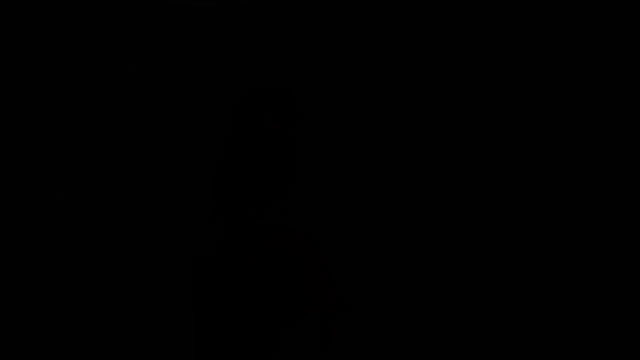 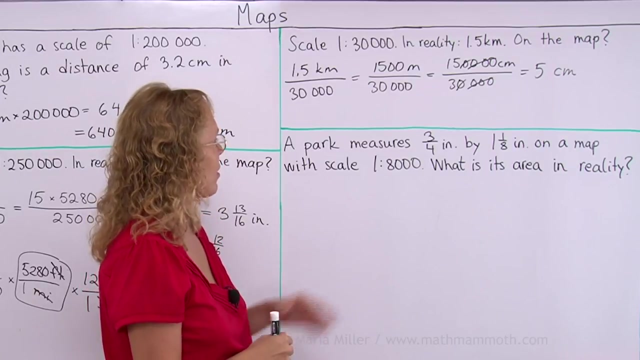 So it is 5 centimeters. Lastly, a park measures 3 fourths of an inch by 1 and 1 eighth of an inch on a map with scale 1 to 8000.. What is its area? in reality, This is a rectangle. 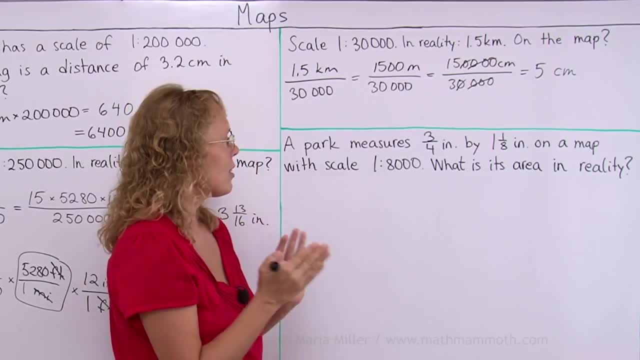 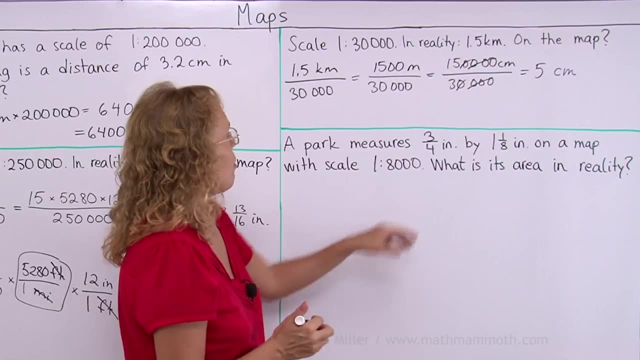 This is a rectangular park, and so to calculate its area, we of course need to find its length and width in reality and multiply those two. We are going from the map to reality, so now we will multiply. We need to make this longer or bigger. 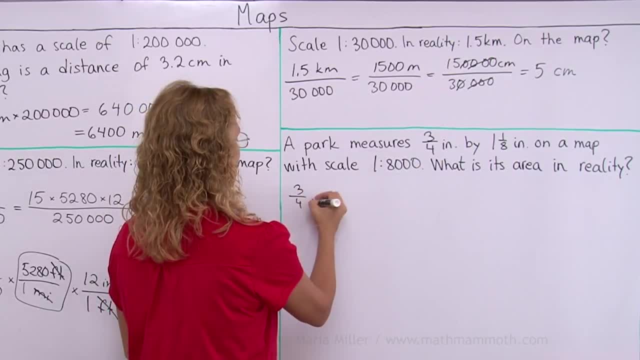 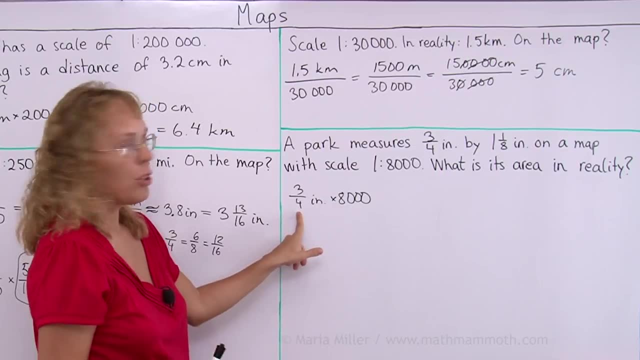 3 fourths of an inch times 8000.. Okay, You can use fractions if you want, Or you can use a decimal number. Just put 0.6.. 0.75 times 8000.. This time we can use the fraction too, because it ends up being 3 times 8, which is 24.. 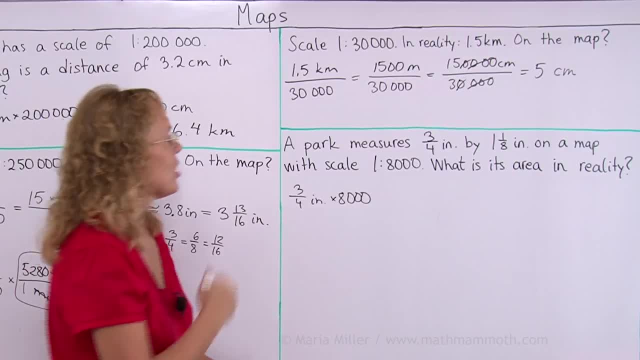 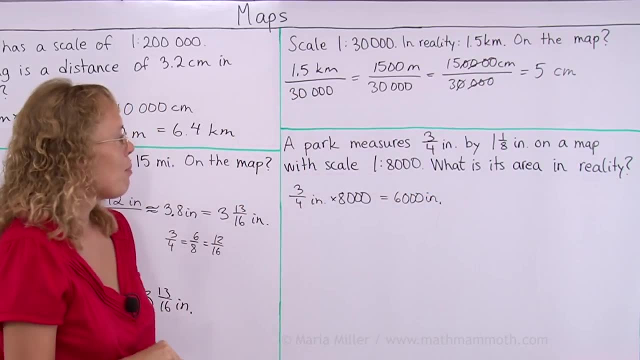 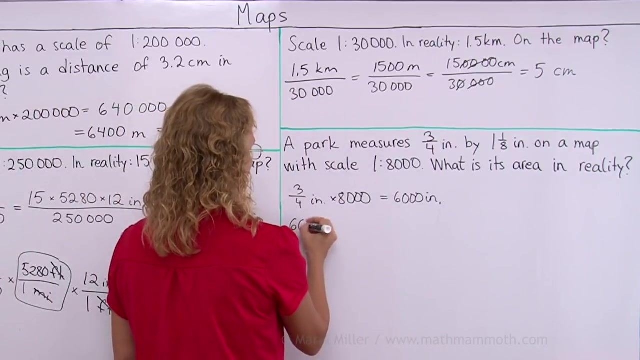 Divided by 4, which is 6.. So this is exactly 6000 inches, But for the park you of course want that in feet or miles, So we need to convert that- still 6000 inches Divided by 12 to get it in feet. 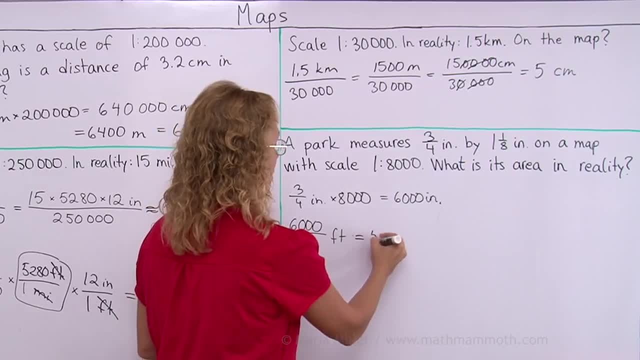 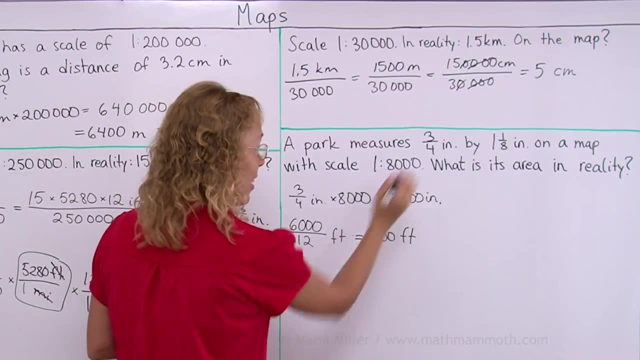 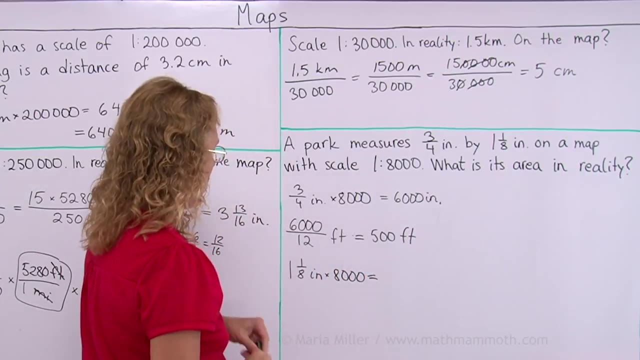 Okay, And that is exactly 500 feet. I have some easy numbers this time, Even though I chose fractions. Okay, and then the other dimension, 1 and 1 eighth of an inch. Here I would have 9 eighths of an inch. 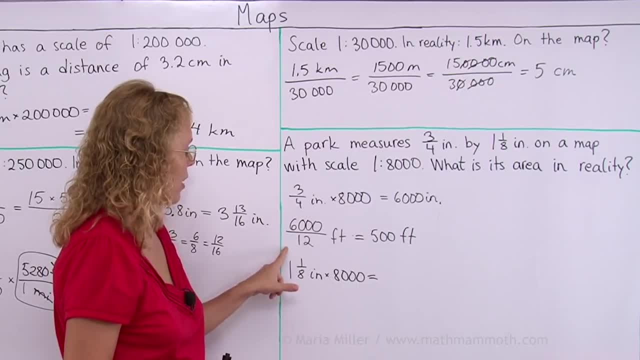 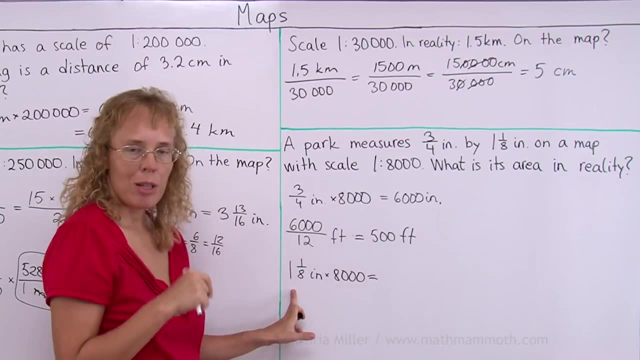 9 eighths, And so I get 9 times 8000 divided by 8.. So that is exactly 9000.. Or you can use a decimal: 1.125 times 8000.. So we will get 9000 inches. 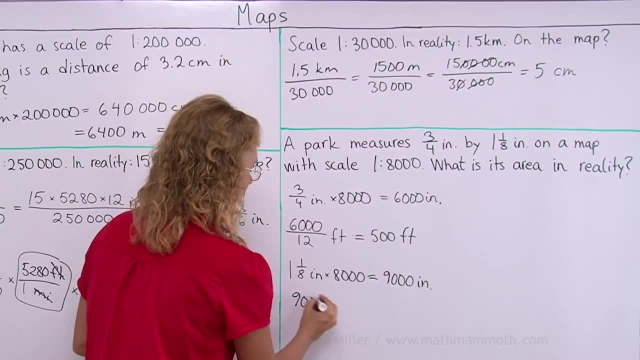 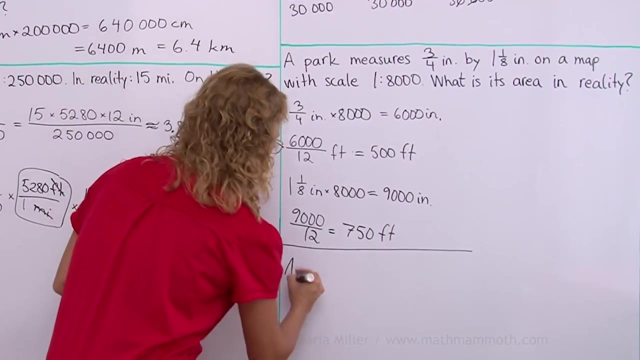 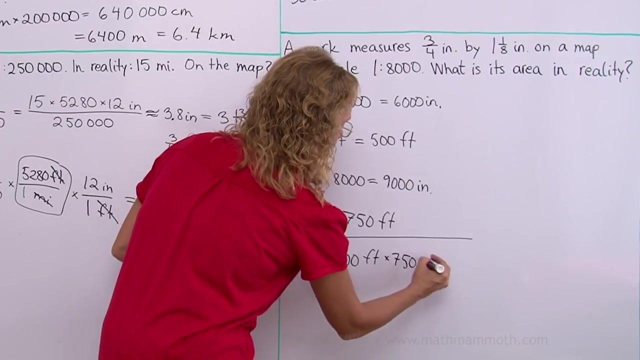 And then we need to do the same as far as finding it in feet. Divide that by 12. And that is 750 feet. Okay, And of course, now all we need to do is just multiply those two to get the area 500 feet times 750 feet.